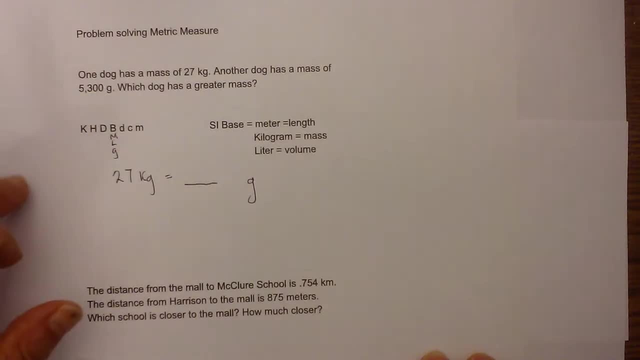 an SI base but it's kind of generally accepted for volume. Okay, I wanted to get that out of the way. So let's convert the 27 kilograms to a gram. So I'm going to put a check where we start and an X where I need to go to, and that is gram And we're going to put the arrow. 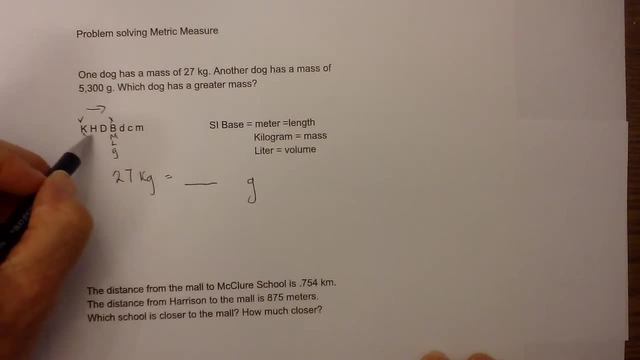 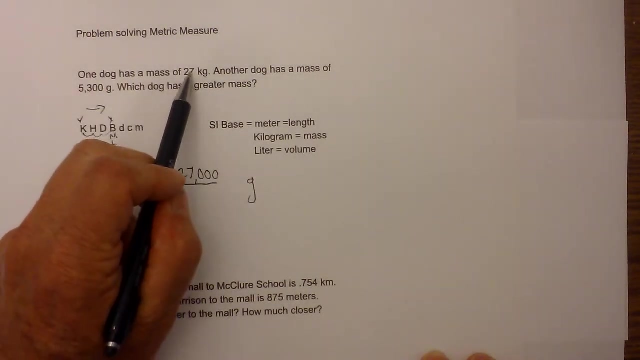 on the check and we're going to go from the check to the X and it is one, two, three, So we need to move the decimal three places to the right. So there's one, two, three, So it is 27,000 grams, And so 27,000 grams is larger than 5300 grams. So the one dog we'll 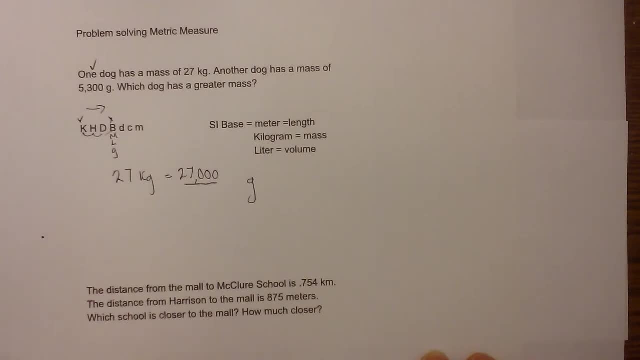 call it. the one dog is indeed has a greater mass. Now, if I wanted to do it the other way, we could go: 5300 grams equals how many kilograms? And we start here with the check. I'm going to go. King Henry died by drinking chocolate milk. And we're starting here because remember. 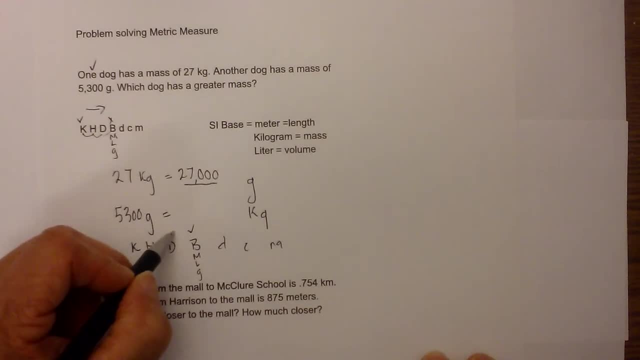 this is meter, liter or gram, And we're going to go to the kilogram in this direction. So I'm starting here and I'm going in this direction. three, So there's one, two, three So that becomes 5.3.. 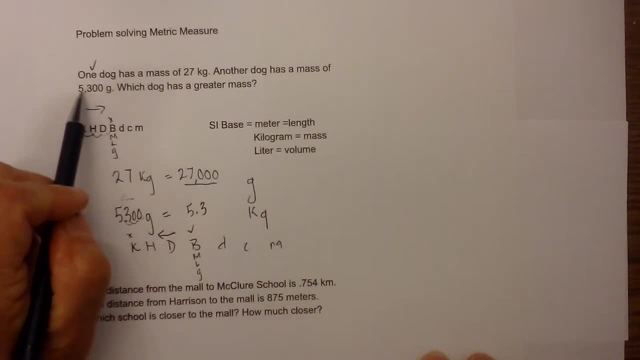 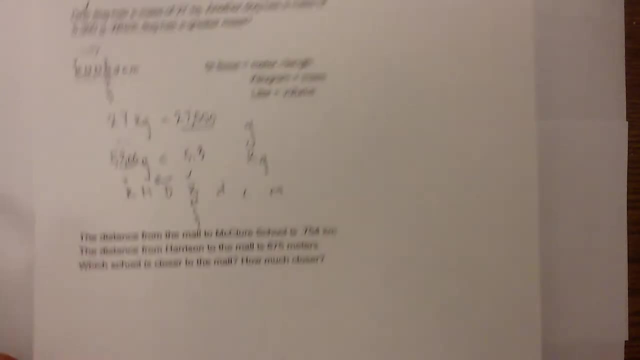 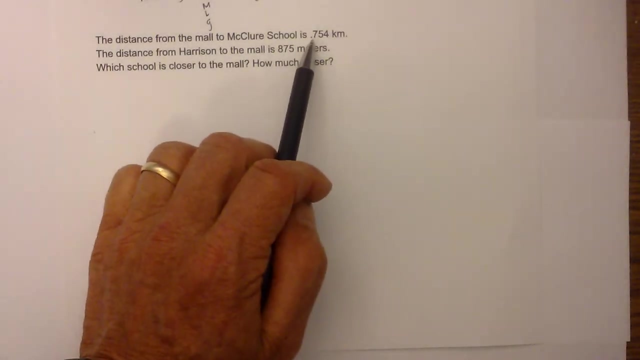 Kilograms And again, 5.3 kilograms is smaller than 27 kilograms. Okay, You can do it either way. So let's quickly move on to our next one And in this particular example it says the distance from the mall to McClure score is .75 kilometers. Distance from Harrison. 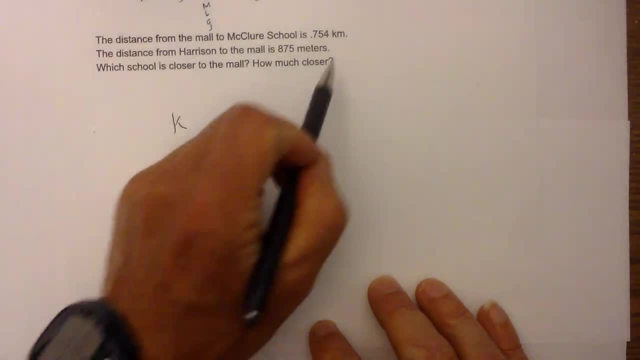 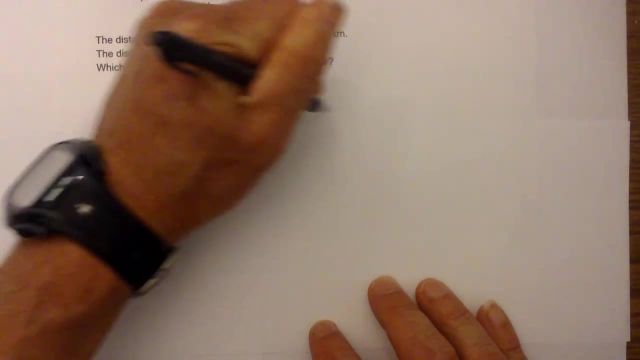 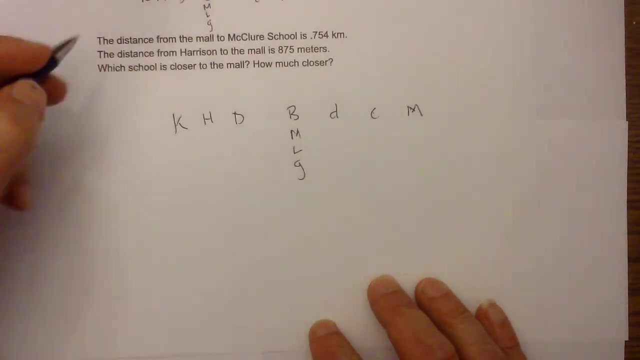 to the mall is 875 meters. So I'm going to convert from kilometers to meters. So I've got King Henry dyed by drinking chocolate milk. meter, liter gram. I'm going to start at kilometer, I am going. 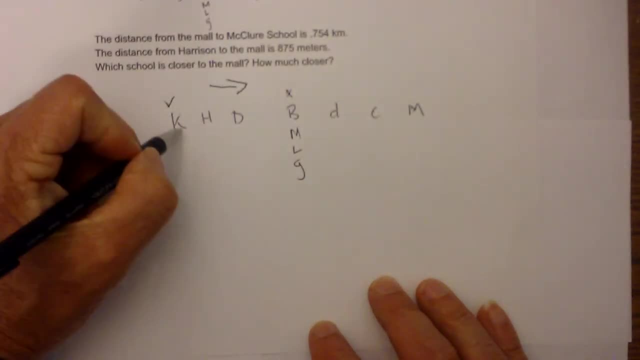 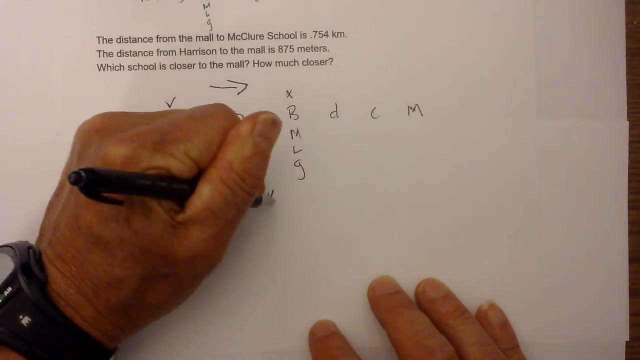 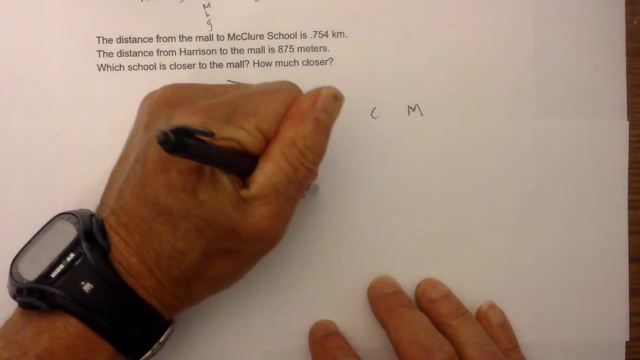 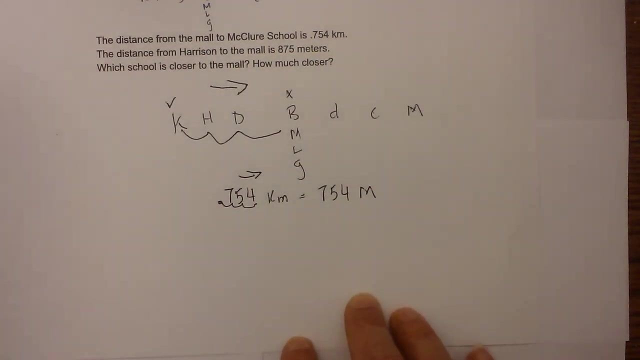 to meter. I will go in this direction: 1,, 2,, 3.. So I am at 7.54 kilometers. I'm going in this direction: 3.. So that equals 1,, 2,, 3. So that becomes 754 meters. Okay, 754 meters. So therefore.